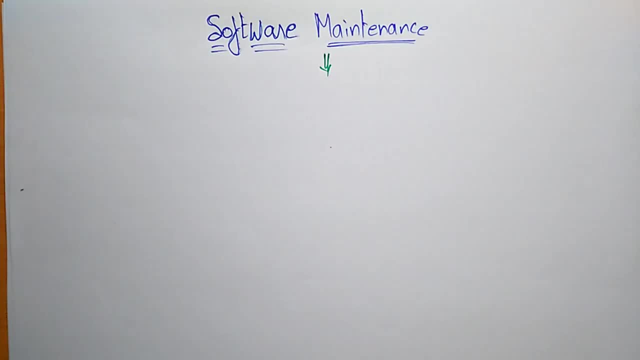 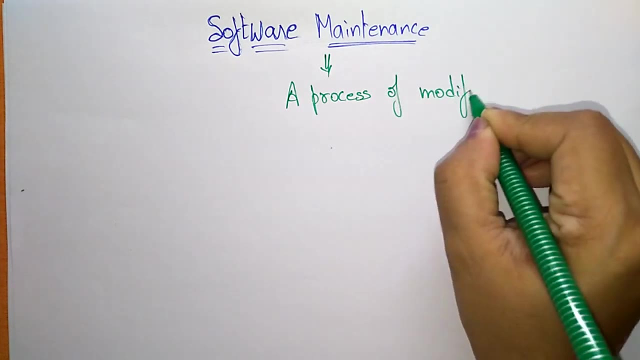 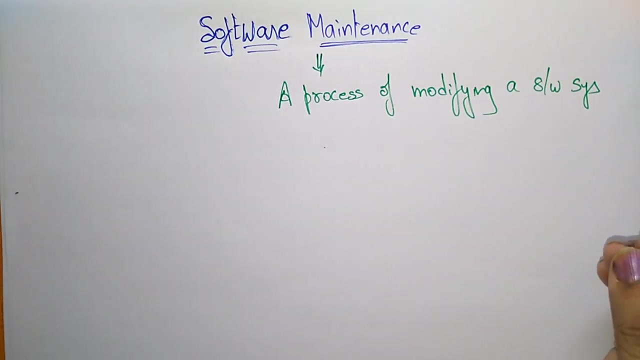 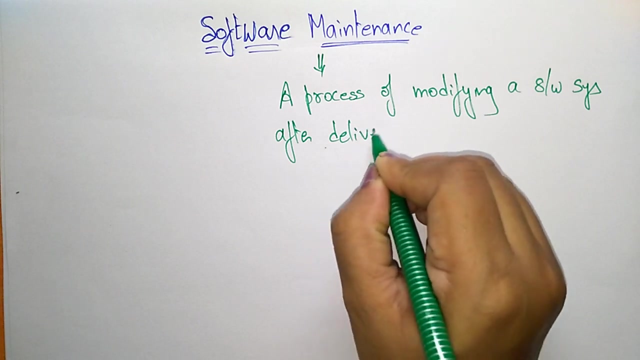 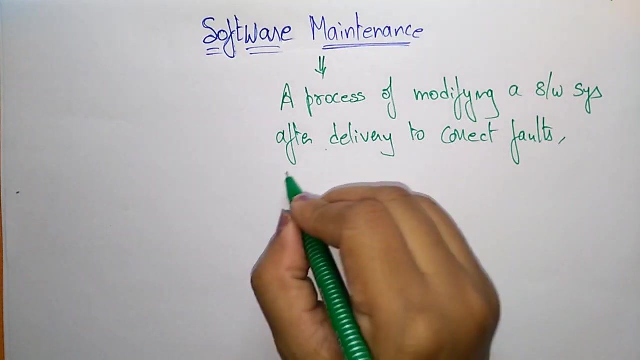 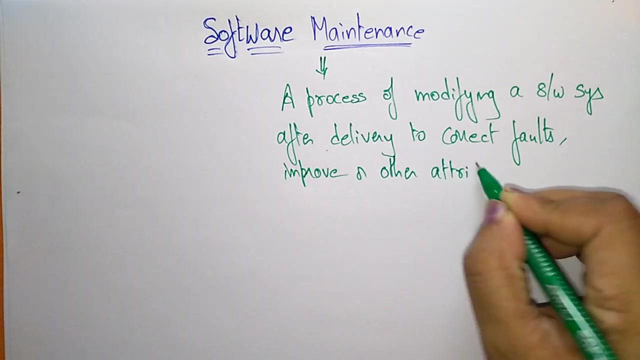 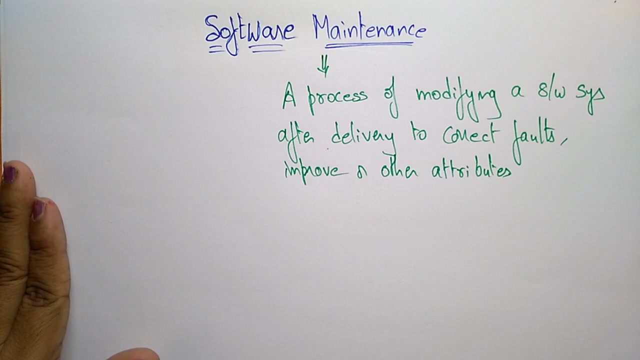 Actually the software maintenance is a process of, it is a process of modifying, modifying a software system. It's just a process of modifying a software system or a component after delivery, After delivery, to correct faults, Improve or other attributes. So why we require this maintenance? Is it necessary after delivery? Is it necessary to maintain the software? Yes, So a process of modify a software system. So means after the delivery of the software product, some the customers need some more, some more modifications to that product. whatever already delivered means I'm adding the extra features. So or to correct the faults, If any fault. 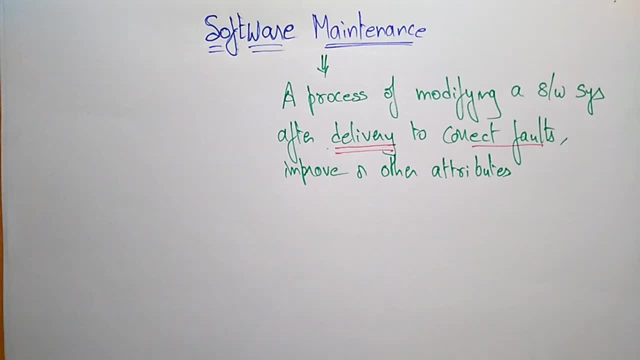 Also after the delivery. that false has to be covered. or to improve the system performance means by adding some more features and by adding some extra services to the product. So this all comes under the maintenance. So all these points or comes under the software maintenance. So what is the difference between the software product and software maintenance? is both of the same? Okay, software product. 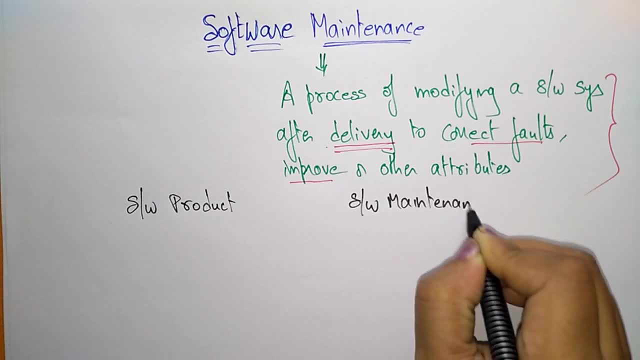 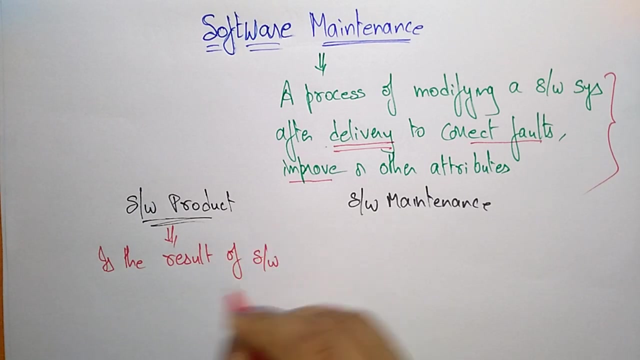 The software product is nothing bad. It is a result of a software development. A software product is the result. whatever we are developed, So that gives some result. So it is the result of software development, Whereas software maintenance is nothing bad. A software maintenance is a results. 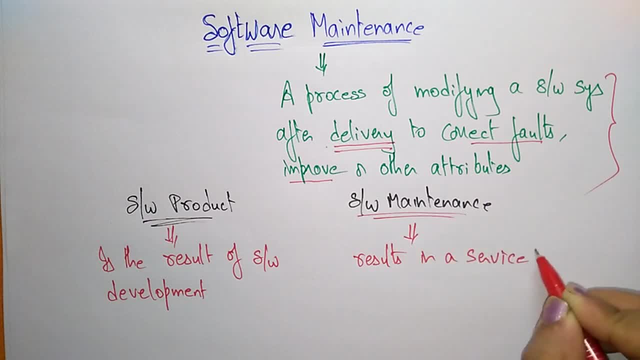 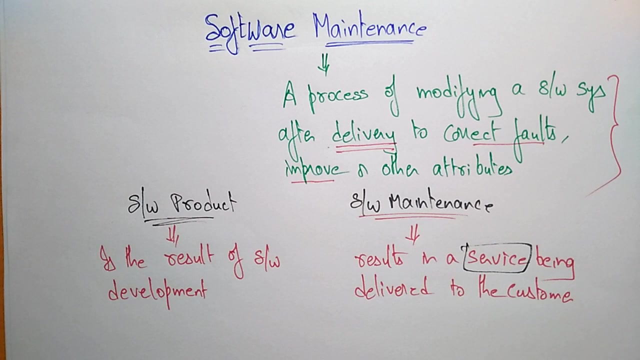 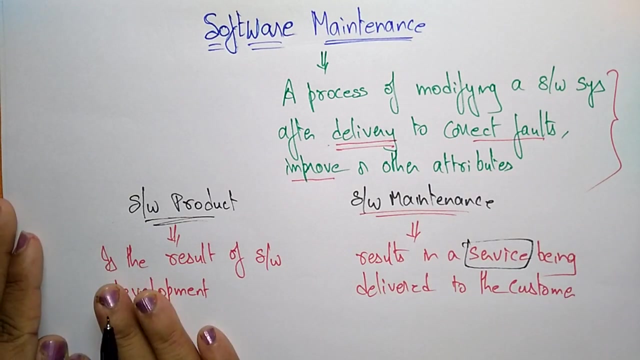 In a service being In a service, being Delivered To the customer. So here the maintenance is nothing bad, It is a service. We are giving a service to the customer by adding some features, by correcting the faults, by improving the efficiency of the system that comes under the maintenance, Whereas a software product is just a result of the software development. 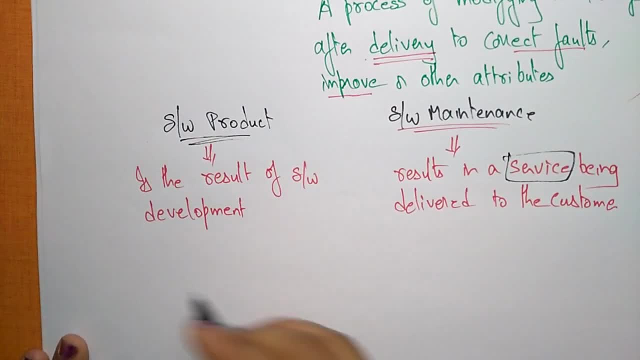 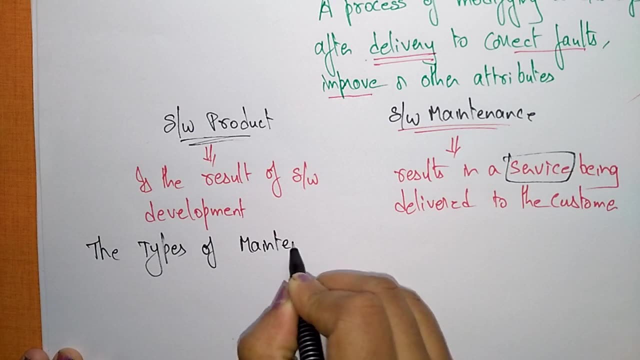 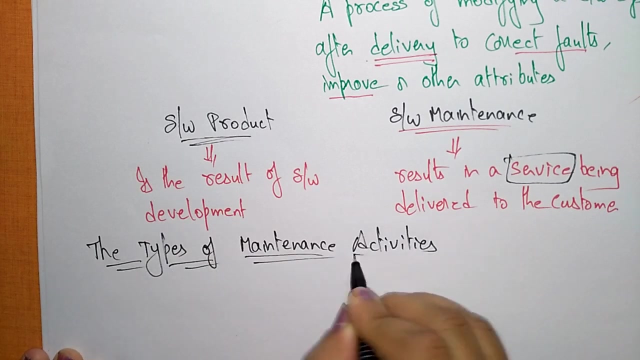 Now let us see the different types of software Maintenance activities, The types of Maintenance Activities. So that is a software maintenance activities. So what are the different types of software maintenance activities? The first one is a corrective. So what is this corrective? When this corrective will come across? 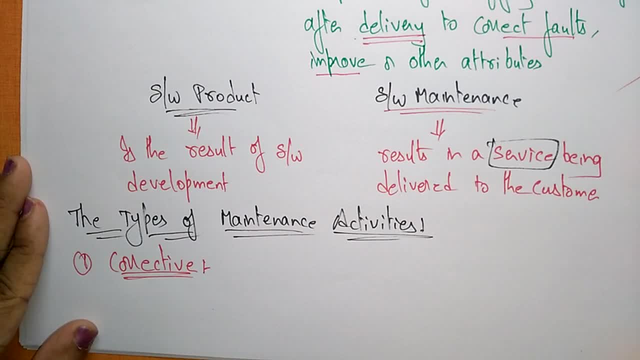 Taking the existing system or taking the existing code and correcting the fault that deviates from its document requirements, that you call it as a corrective. Okay, So actually, whatever the requirements we are getting, means, after the clarification of every means, whenever you have prepared the SRS document. means whenever you've prepared SRS means it is you have to fix to that requirements. 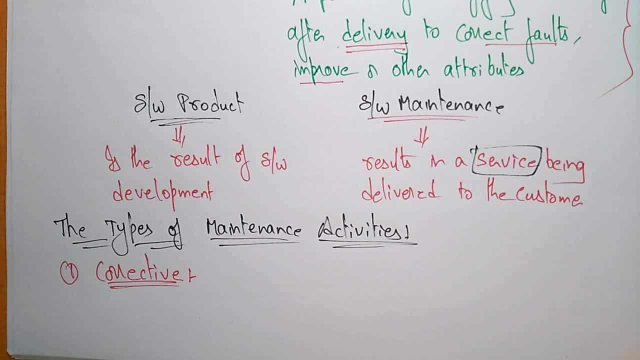 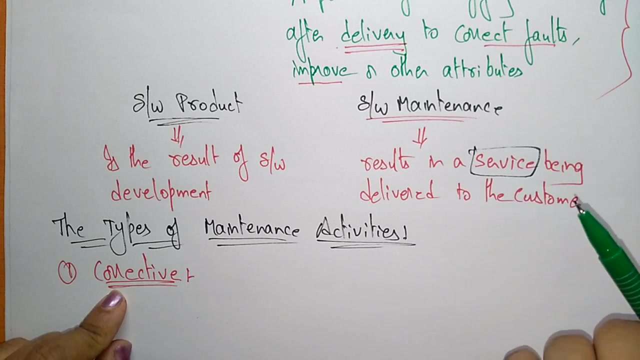 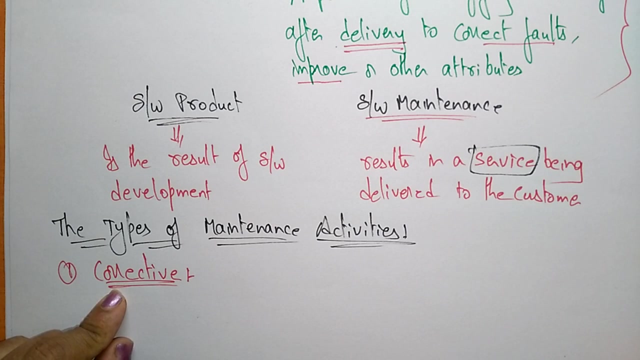 So we will start Implementing the product by seeing the requirement SRS document. So then, what is this corrective? So, when we are doing this corrective in the maintenance, So taking the existing code, whatever we already implemented, just you have to take that existing code and correcting a fault which is deviated from its document requirements means sometimes there is a possible. if you have missed the some points while developing, means you just missed the point. 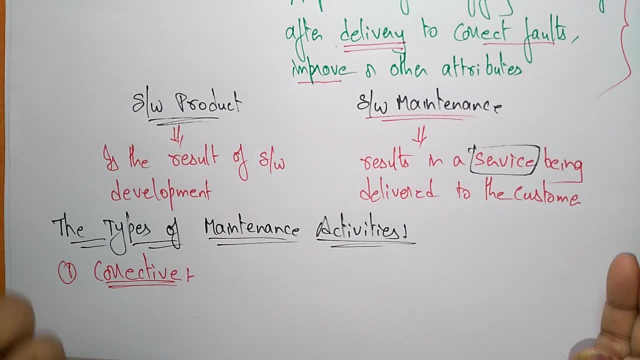 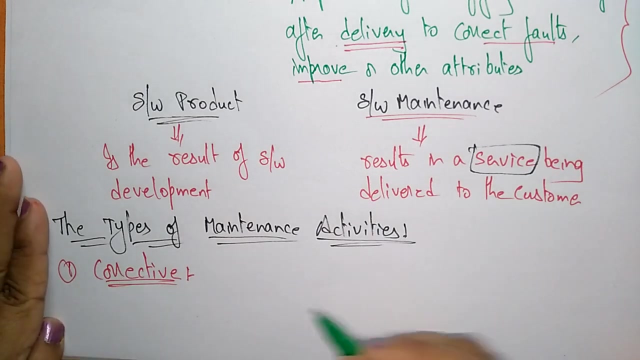 Some activities in the documentation which are the requirement documentation. So with that problem, you just deviated from the requirements so that you have to be corrected. So this is one of the activity: maintenance activity. Let me write that point: taking existing code and correcting a fault. 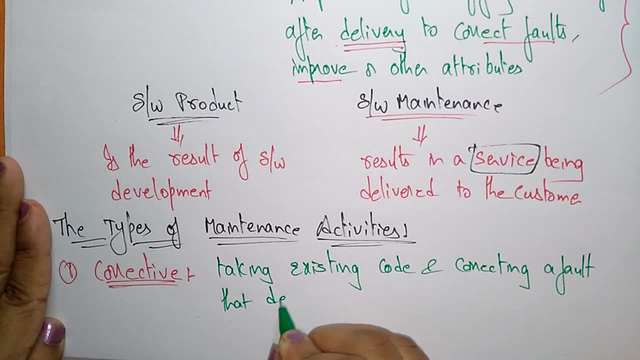 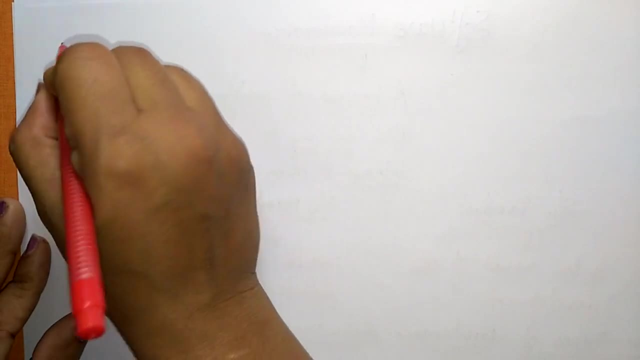 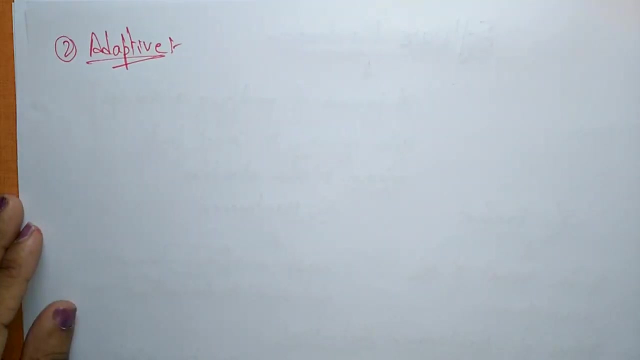 Correcting a fault that deviates. That deviates from its document requirements. Now let us see the second time. So what is the second time? The second type is adaptive. Adaptive is nothing, but you have to take the existing code and adapting it to provide new features and functionality.